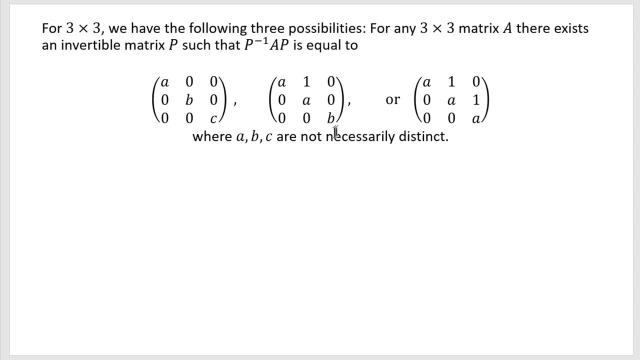 and then a separate number, And still A and B could still be the same or different, And then you have a case where it's the same numbers here, but then you have one and one off diagonal. okay, So these are the three possible cases you can have as Jordan canonical. 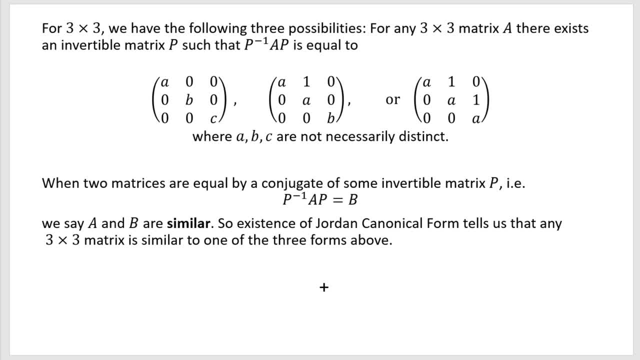 form for a three by three matrix. Now, when you have two matrices equal to each other as conjugating by P versus A, P is called conjugation of A by P, And if that's equal to B, we say A and B are similar. 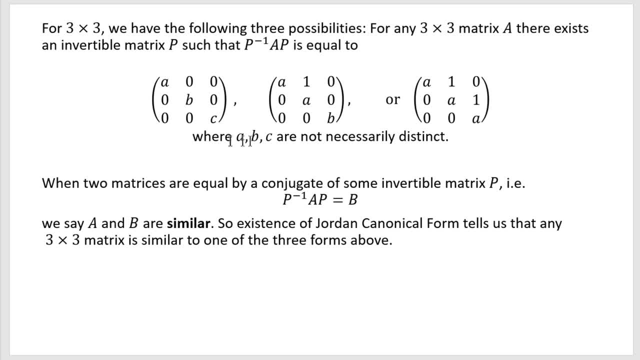 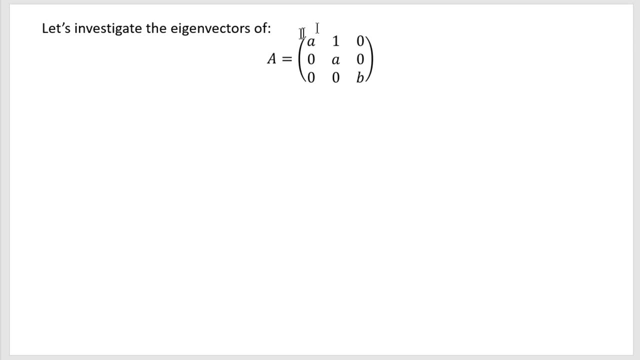 okay, So another way to say this result is to say that any three by three matrix is similar to one of these three matrices. okay, All right, so let's try to investigate the eigenvectors of this one to understand what's going on for such matrices. okay, So? 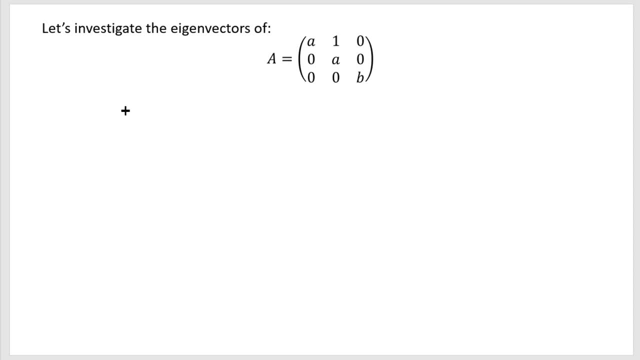 I'm hoping that you already know how to diagonalize a matrix using linearly independent eigenvectors. That will be the first case right here. But we want to investigate what happens to these matrices where it can't be diagonalized. okay For this kind of matrix. you can readily see that if you 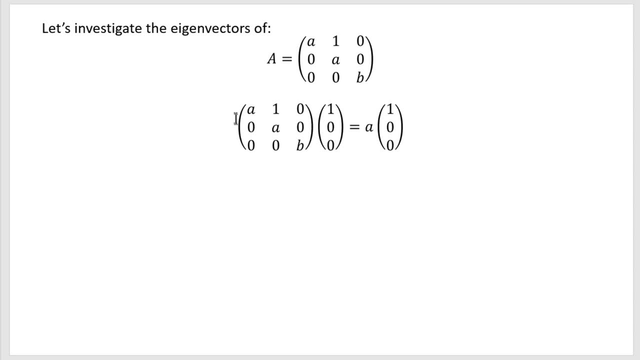 multiply 1, 0, 0, you get A times 1, 0, 0,, same as A times V. So what's an eigenvector? Eigenvector is when you have- A V equals to 2. Capital- A V equals to some number times V. So here lambda is small. 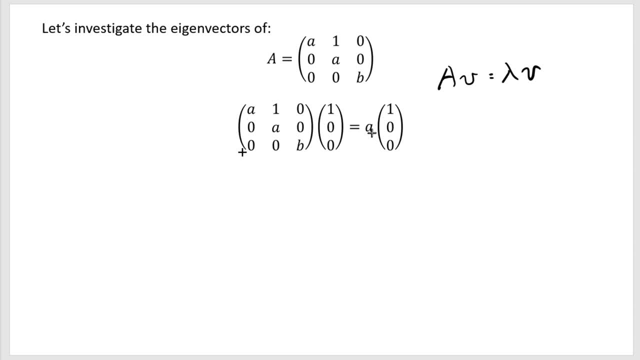 A, and this is the matrix that we're trying to look at. okay, So we see that this is indeed an eigenvector, And likewise you can also see that 0,, 0,, 1, when you multiply it. you. 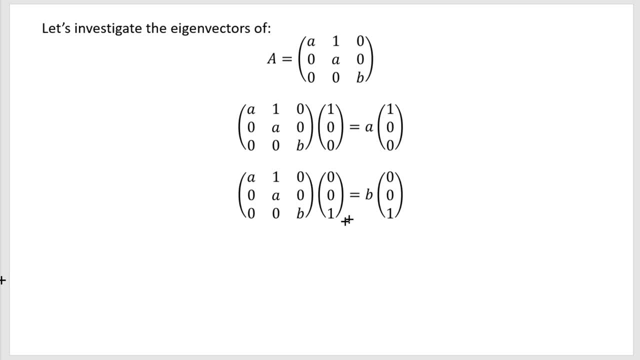 get-. you see that 0, 0, 1 is an eigenvector with eigenvalue B. However, that immediately brings us to question: what about 0, 1, 0,? right For the 0, 1, 0,. what happens is? 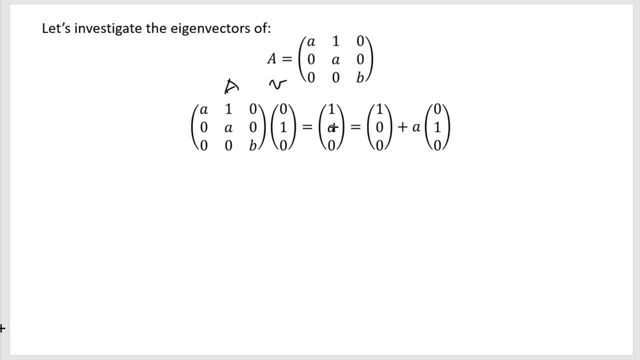 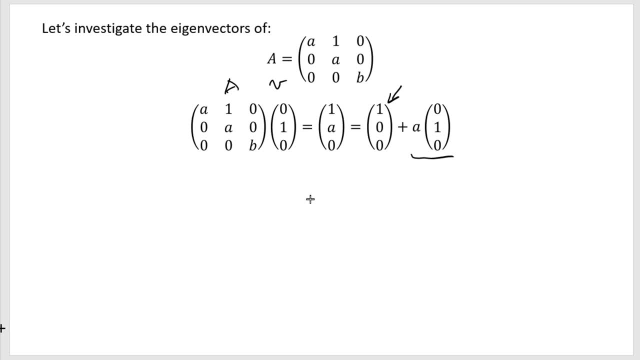 This wasn't there, And then it will be an eigenvector, right. But you then recognize that this is itself an eigenvector. This is not. This is not an eigenvector because it doesn't satisfy the eigenvector equation, but this is an eigenvector. So if we 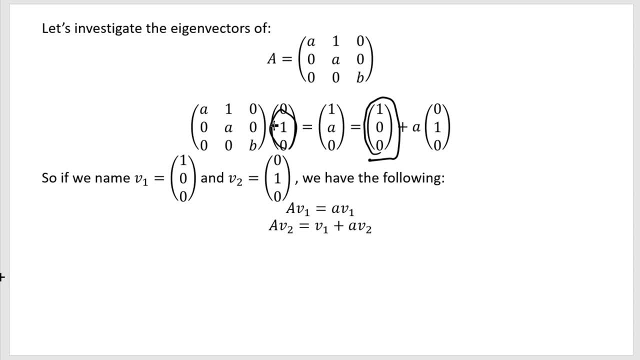 write down the above, call this column vector as V2, and you have A V2 equals to V1 plus A, And often people write this equation in the following format: that the eigenvector equation is A times lambda I. V1 equals 0, that's the eigenvector equation, right. 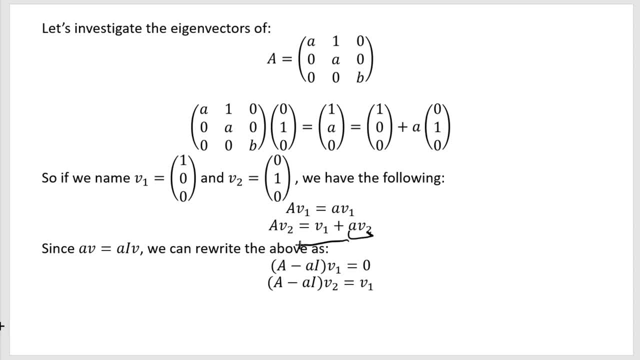 But this one looks pretty similar if you move this A V to the left side and write it as A minus A I V2, V1.. Oh, by the way, if you're wondering how that's possible, just think of it like this: 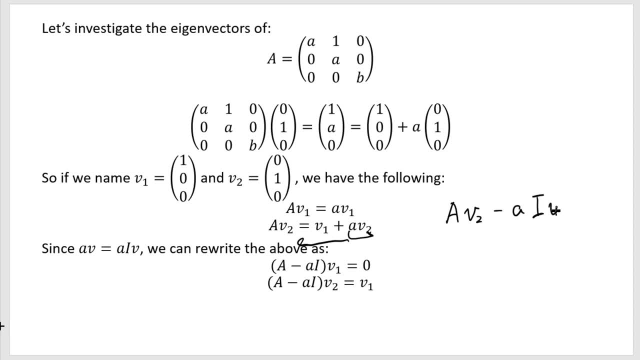 You have A identity matrix. times V2 is the same as V2, so I can move this to the left side and write it like this, And then if I factor the V2 out, you do get A V2 minus A. I equals V1, right. 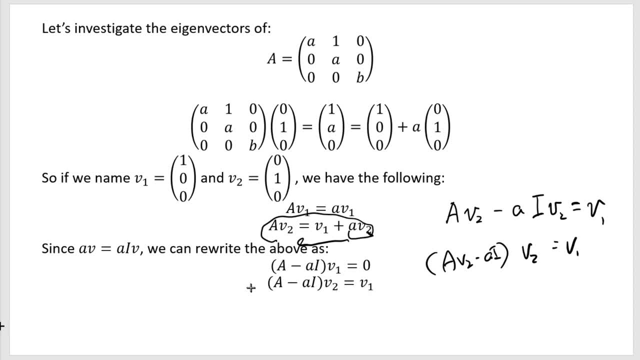 So this equation can be written like this: and this resembles the eigenvector so much that there's a name for that. okay, So there's a name for that. In addition, we see that this means that if you apply A minus A, I twice, applying it once. 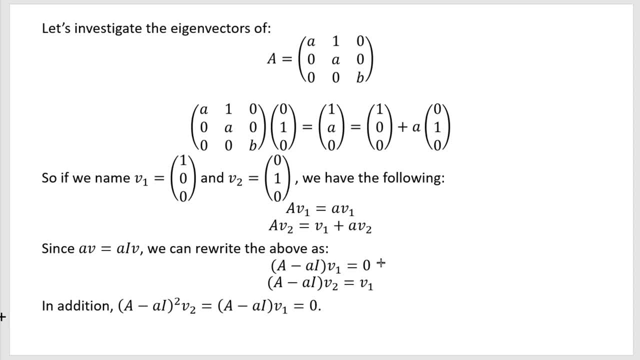 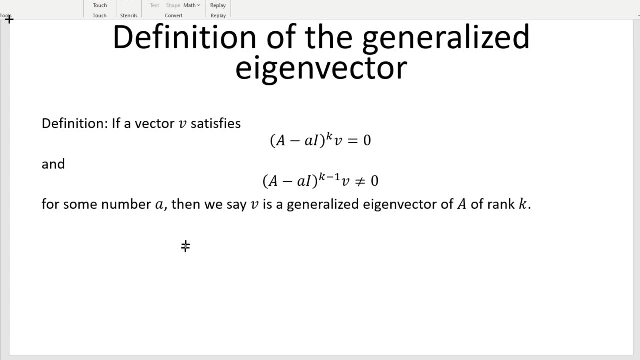 turns it to V1 and then applying it once it kills it. because of the first equation And these two relations are actually pretty important- that you have a name for them. Okay, and the name for that is a generalized eigenvector, okay. 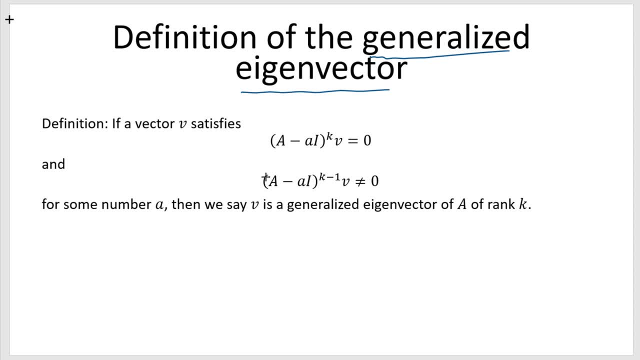 So what's a generalized eigenvector? It's something, it's a vector which satisfies for some positive value of K, that this times V is 0, whereas if you do negative, 1,, if you do 1 less than what you applied before, then. 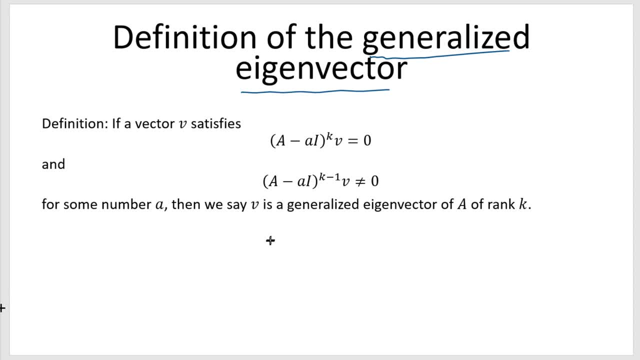 it's non-zero. Okay, So by default, any eigenvector is already a positive value. Okay, So if you do 1 less than what you applied before, then it's non-zero. Okay, So that's a generalized eigenvector, because that's for the case when K is 1.. 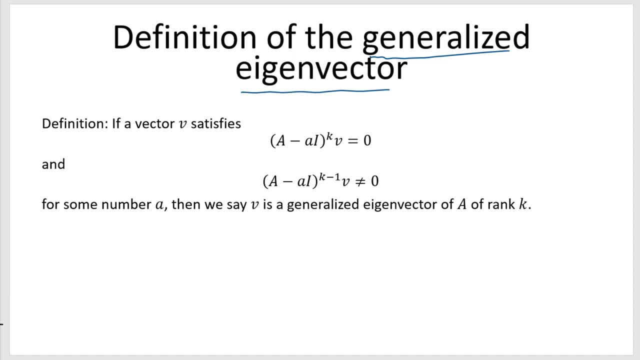 Remember that eigenvectors are not allowed to be 0, so that's what the second condition is saying. And then in the previous example we have that applying A minus A I of V2 is V1, then we say it forms a chain. 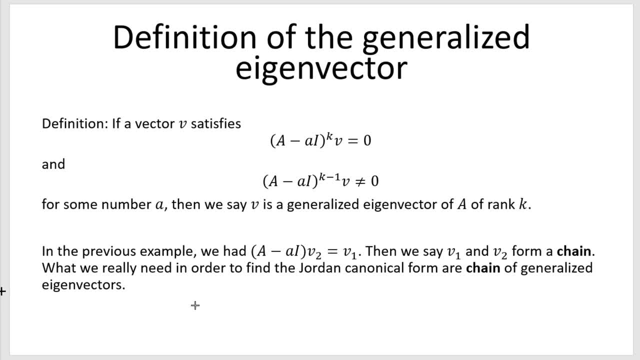 So this is a chain of length 2, but you could have chain of any length. So, for example, you could have something like this: You could have something like A minus lambda I of say, V4 equals to V3, and then this: 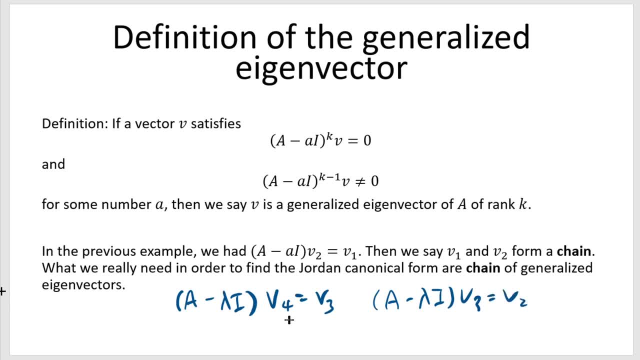 times V3 gives you V2, and then A minus lambda I times V2 equals to V1, and then finally, A minus lambda I. V1 is 0, because V1 itself is an eigenvector, And so in that case we have a chain of generalized eigenvectors of length 2.. 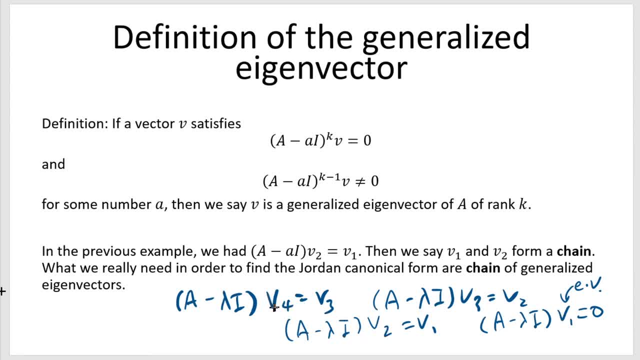 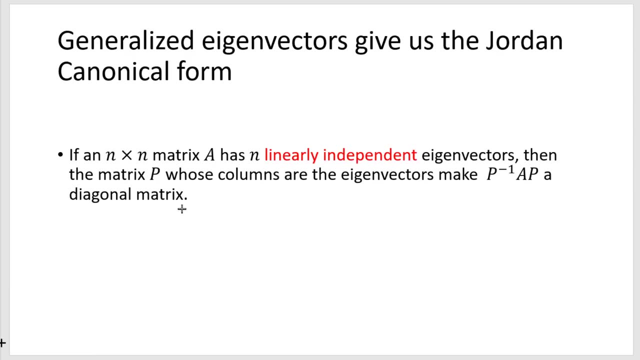 Okay, So that's a generalized eigenvector. Okay, And we will see that in order to get the Jordan canonical form, you need to find these generalized eigenvectors. Okay Now, so recall that if you have n linearly independent eigenvectors for an n by n matrix, 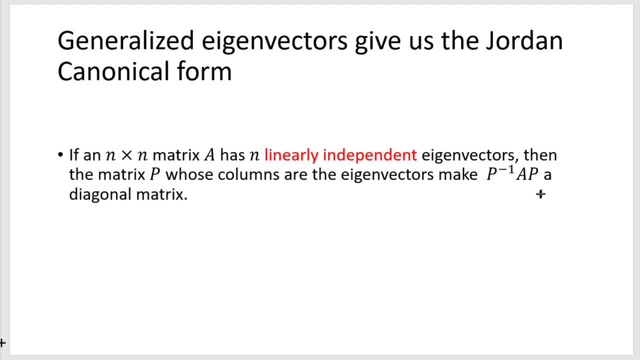 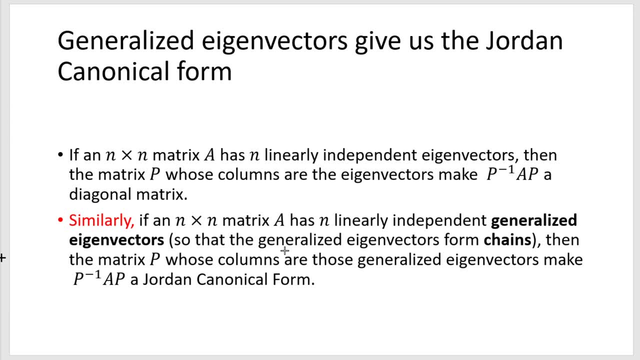 then you can diagonalize it. The matrix is similar to a diagonal matrix, So I'm going to assume that you know, Okay. And then, similarly, if you have generalized eigenvectors, so in the form that they form chains, then you can build this matrix P whose columns are those generalized eigenvectors. 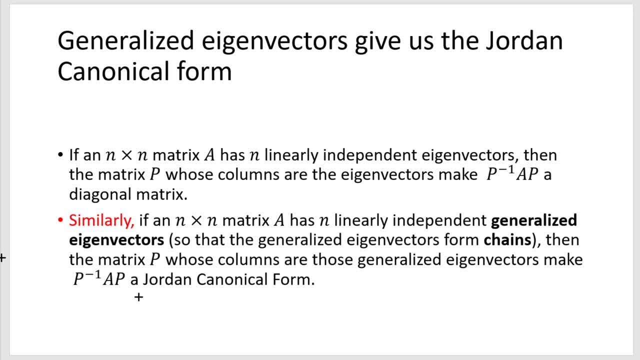 and make P inverse A P a Jordan canonical form. Now I don't want to give you a proof of this. Rather, I'm going to give you a demonstration of how it works for a 3 by 3, and when you see it you'll kind of see how the mechanics work. 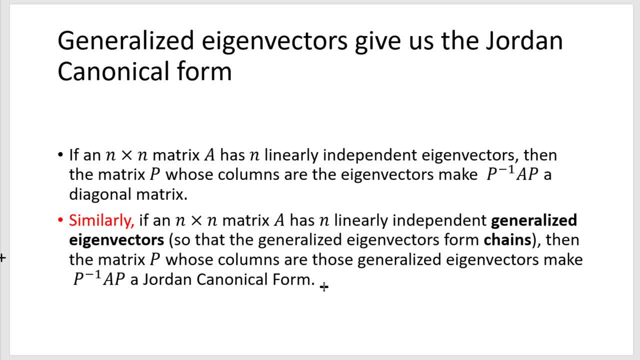 Okay For the actual proof. it requires a lot more work, So I would suggest that you just have patience and read the books, But here, if you see how it works, you will get a much better understanding when you see the proof. 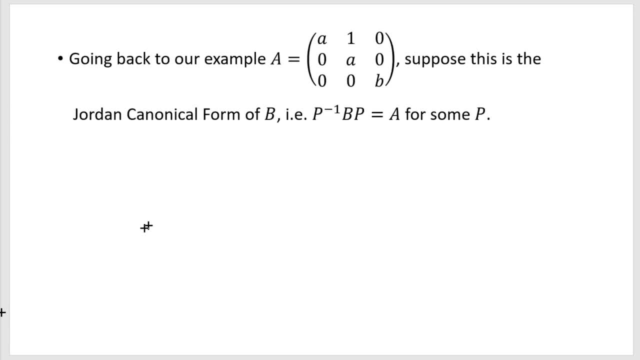 So hopefully don't turn off the video, Just keep going. Okay, All right. So, going back to our example, we found out that there's this V2, whose A minus Ai gives us a 2. Okay, Okay. So let's say that there's a matrix B whose Jordan canonical form is this one: 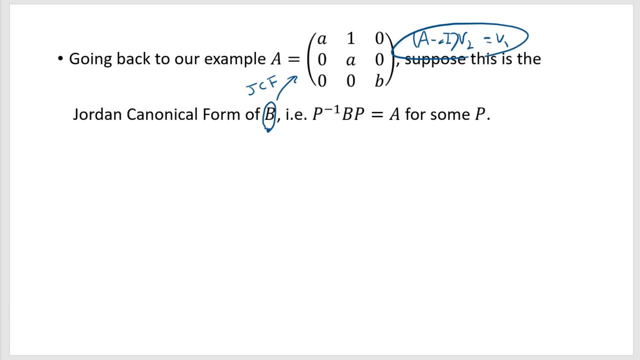 Okay, Jordan, canonical form is this one. In that case you can rewrite A V1 equals to A V1 as P inverse B. P V1 equals A V1, and then you multiply P both sides. Then you get this, because P and P inverse cancel. so you get this on the left side. 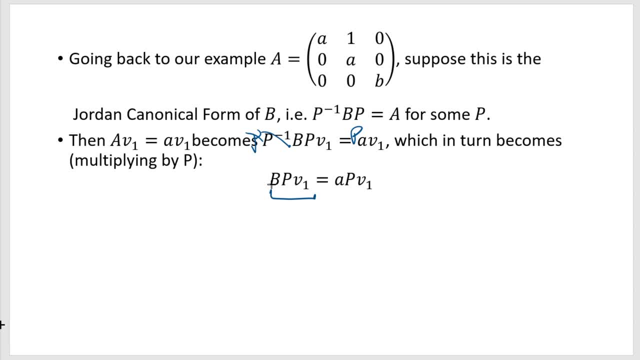 and constant can be pulled in front, so you get B, P V1, A P V1.. And what this means is that these two vectors are actually eigenvectors of B. Okay, So what this shows us is that actually similar matrices have the same eigenvalues and also: 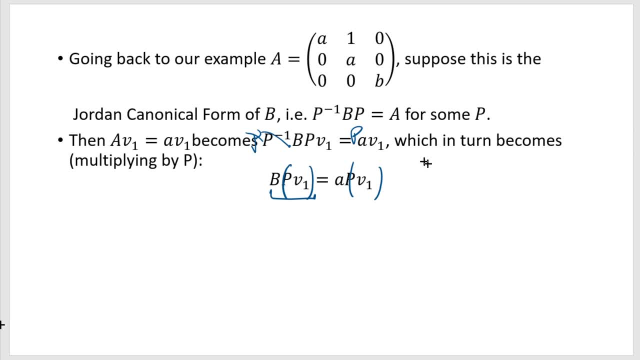 you can convert one generalized eigenvector to another. I didn't talk about generalized eigenvectors, but even for generalized eigenvectors, recall that This is the equation between V2 and V1, and if you do the same process, you get the exact. 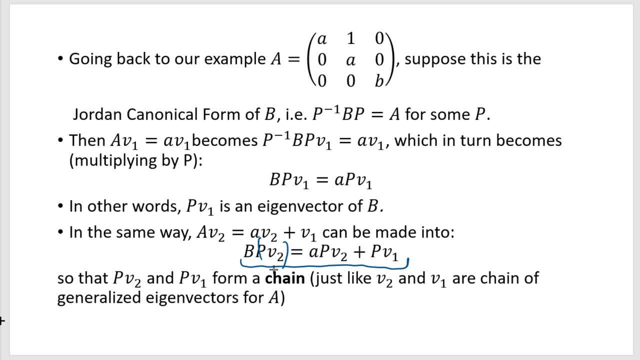 same thing, which says now: P V2 is a generalized eigenvector. Okay, And this is nice, because if some matrix B cannot be diagonalized and its Jordan canonical form is something that has a 1 like this, then we should be able to find a generalized 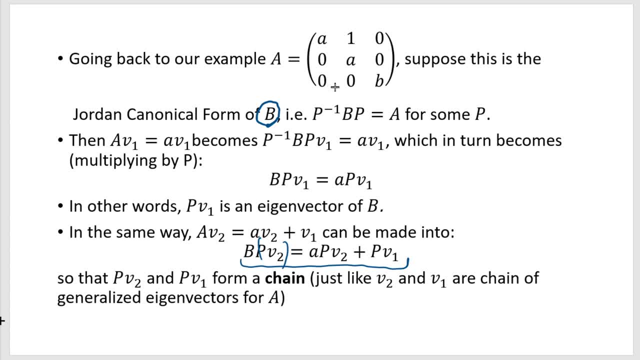 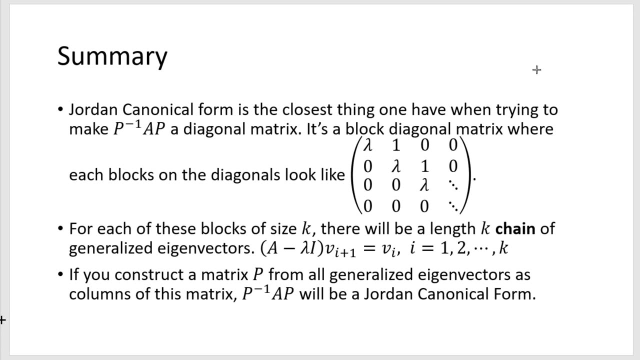 eigenvector chain of length 2, and that's going to help us to put it into this form. Okay, All right, So here's the summary. I didn't give the full proof, but with the demonstration immediately following, you will. 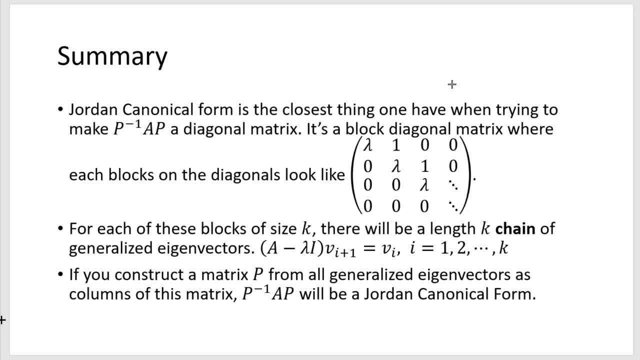 kind of understand what's going on. Okay, So what's a Jordan canonical form? It's not a diagonal matrix, but it's a block diagonal matrix where you have these things on each side. Okay, So you can see that the diagonal matrix is the same as each diagonal block. 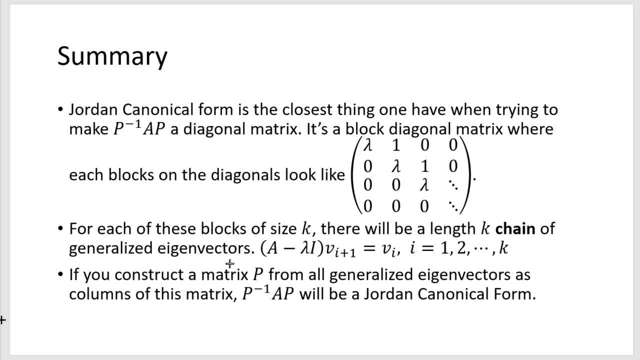 Okay, Block diagonal matrix on the diagonal. Okay, All right. And then there are something called generalized eigenvectors of length k, and if you find all the generalized eigenvectors of this matrix, you can construct a matrix P with these generalized 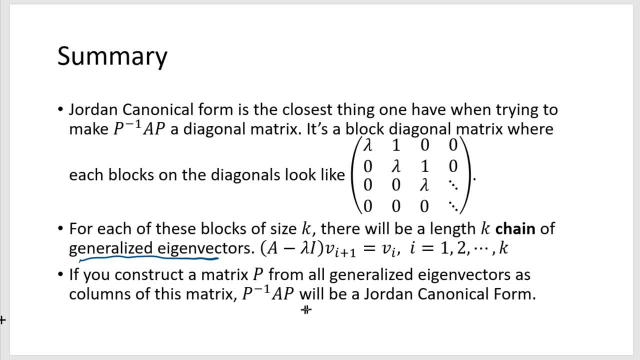 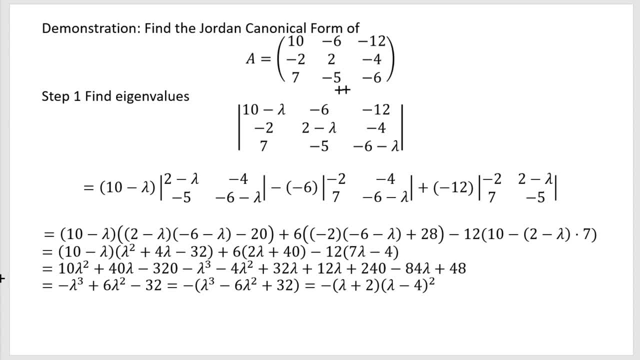 eigenvectors and you will end up with a Jordan canonical form. Okay, So let me give you the demonstration. So here's the sample matrix. I want to find the Jordan canonical form of this, and you first have to find eigenvalues. 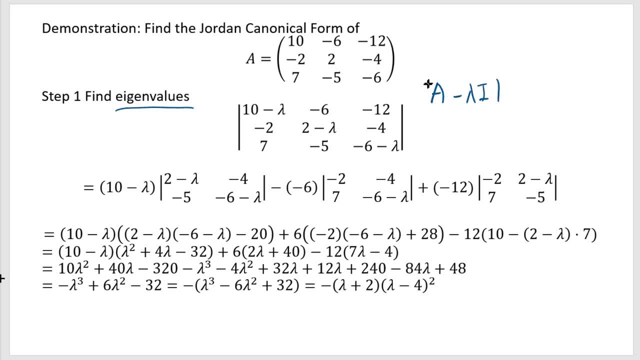 Of course eigenvalues. you do A minus lambda I. You have to take the determinant equal to zero. That's exactly what I'm doing. and when you calculate the determinant you need to do row expansion. so I take this times the minor matrix, then minus the second times the minor. 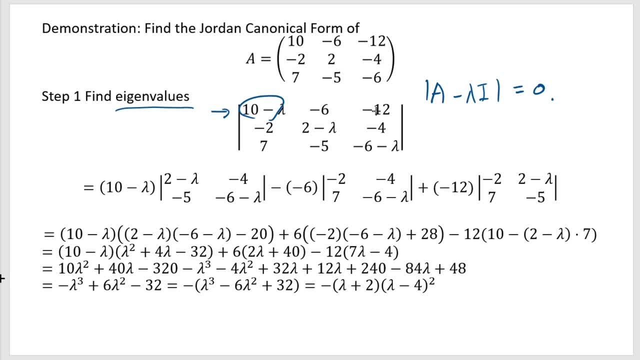 matrix. This is when you delete the column and the row, so you get these four as a minor matrix and the sign goes plus, minus, plus, Okay, And then after that you get some algebra, some bit of a long calculation, but after: 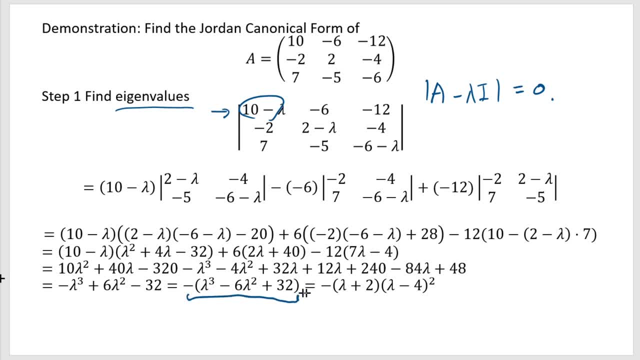 you get the following, get the final form, then you can use something like, say, synthetic division, synthetic division, And then check that say negative 2 solves it 1, negative: 2, add the negative: 8, positive. 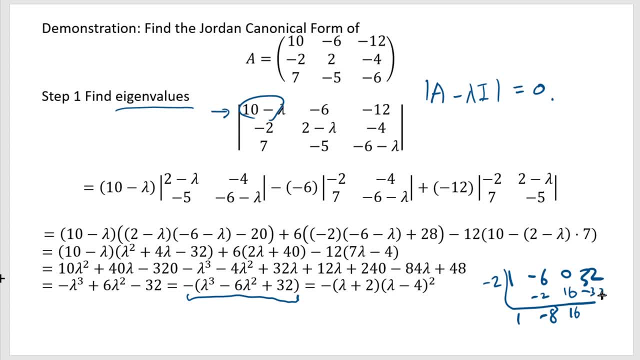 16, positive 16,, 16 times negative 2 is negative 32, and you add them you get zero. So if you know synthetic division you can factor this. If you don't, please review how to do the synthetic division to factor a cubic polynomial. 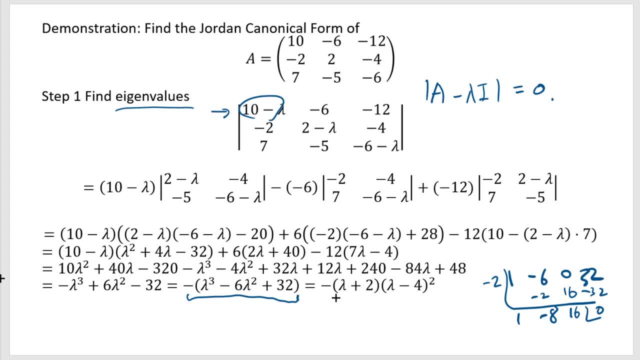 Okay, So you have that And then after that you can, If you further factor, When this is x squared minus 8x plus 16, you can factor that to get x lambda minus 4 squared. So we see that the eigenvalues are negative 2 and positive 4.. 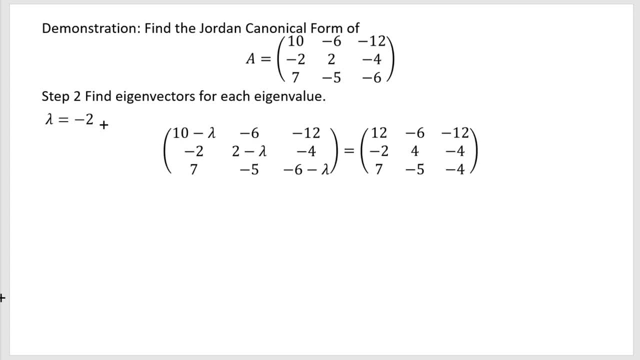 Okay, So that's step one. Now step two: what you do is, for each eigenvalues, find the eigenvectors. So you plug in negative 2 into this, a minus lambda i, and you get this vector. And an eigenvector is when you multiply it. 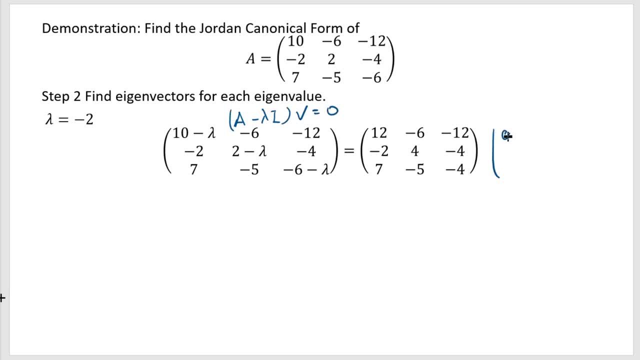 This times v equals to zero. So you're trying to look for some matrix column vector which this times this equal to zero, which is not so easy to see. It's hard to figure out which one will work, And in that case a nice thing to do is to do the row-reduced echelon form of this thing. 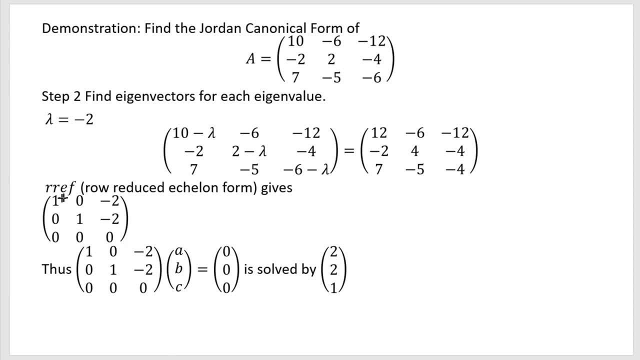 Okay Now, This is basically obtained by using Gauss elimination. If you don't know what Gauss elimination is, you should also review that too. And instead of spending time doing this, I just want to demonstrate, So I'll just use a calculator. 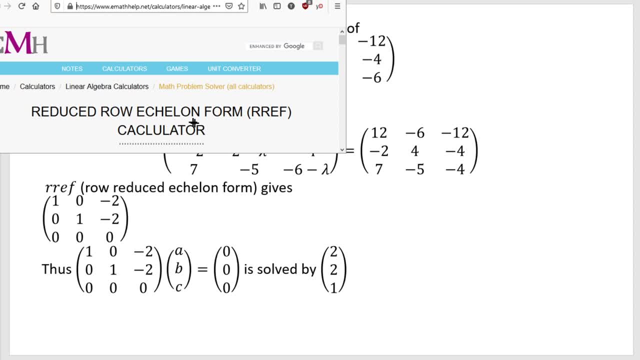 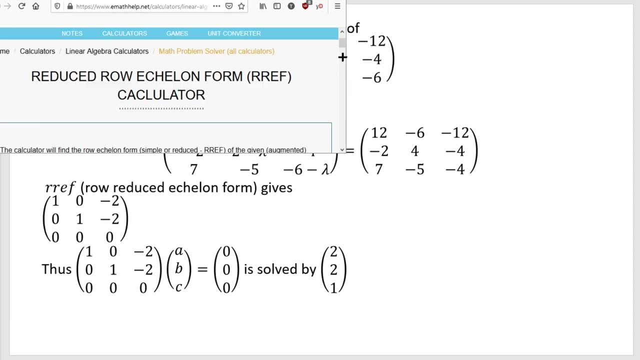 So there's this online calculator for reduced row echelon form calculator, RREF. You also have this functionality on your TI-80.. Okay So, Okay. So I'm going to use the TI-84 and other calculators as well. 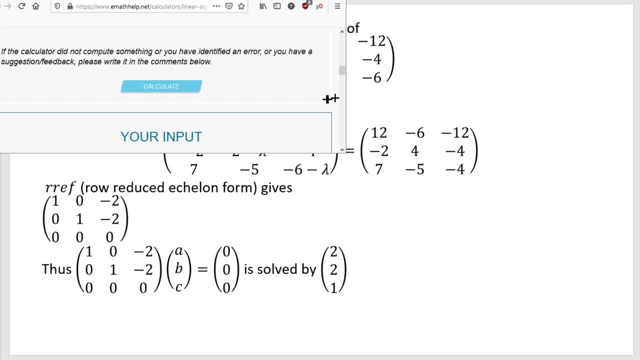 So I plug these numbers in here and I click calculate, and this website actually gives you not only the final form but how you actually get it. Okay, Alright, I just googled this, So you can just google it. reduced row- echelon form- show steps, and then you'll find this. 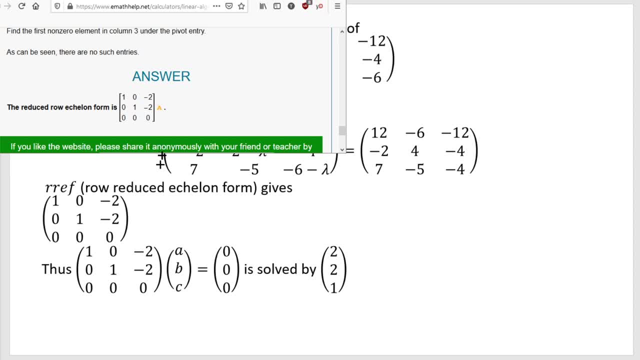 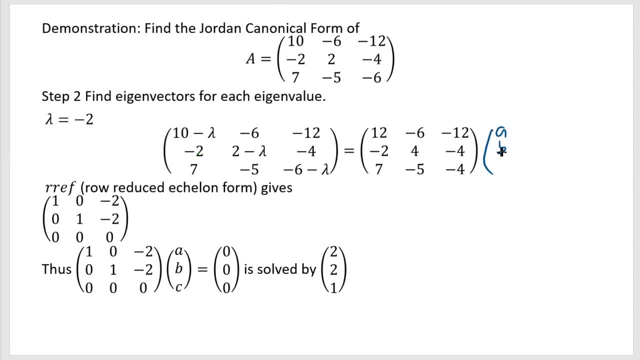 or other. There are other websites too. Okay, So you get this. And what does that mean? That means, see, when you try to solve this, ABC equals to 0, 0, 0, Gauss elimination tells us that it will be same as solving this instead. 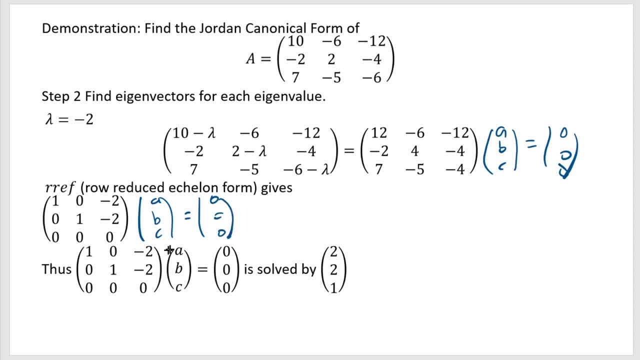 Okay, So that's what I'm doing. But if you actually write out what that means, it's A minus 2C equals to 0, because it's 1, 0, negative 2.. So that means B minus 2C equals to 0.. 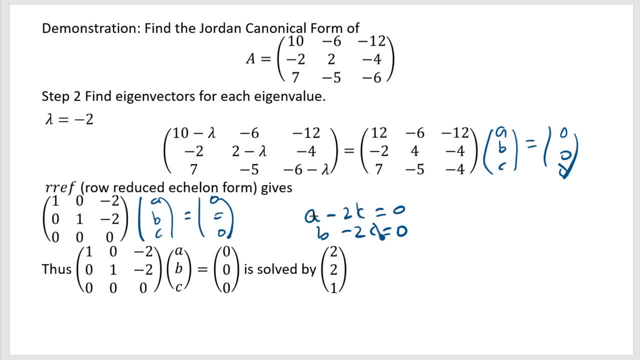 So that means, if you say C is 1,, then B will be A, A will be 2, and B also will be 2.. So this is one solution. Okay, So that's your eigenvector, for lambda equals to negative 2.. 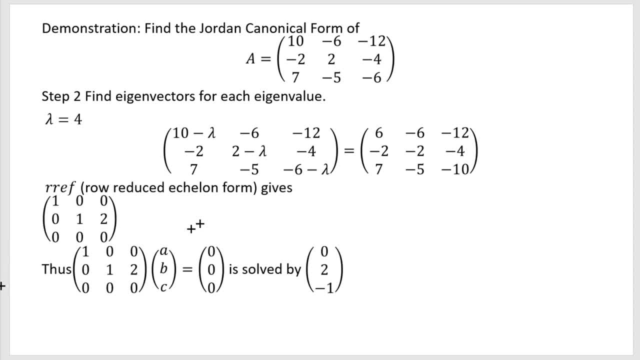 Alright, So you can do the same thing for lambda equals to 4.. I'm using the row reduced again, and this means that A has to be 0, and B plus 2C has to be 0 as well, So this must be negative 2.. 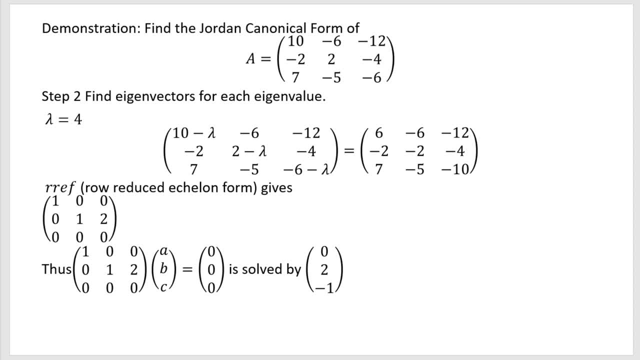 Okay, So this is negative 2 and negative 1.. Alright, The problem is this is: see, this is rank 2.. So there's only one eigenvector, non-zero eigenvector, that is, that comes from lambda. 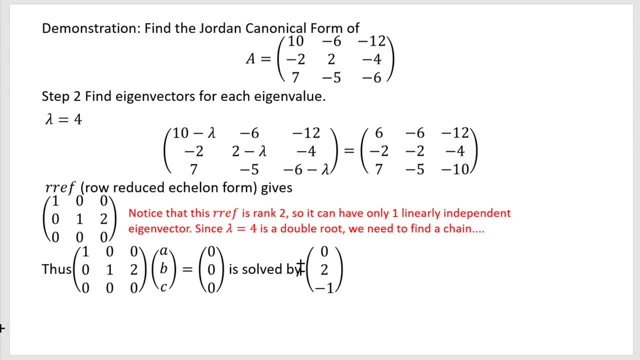 equals to 4.. All the other ones will be linearly independent with the one that we just found. But because this is a 3 by 3, having just two vectors- one for lambda equals to negative 2 and one for lambda equals to 4, it's not enough to diagonalize. 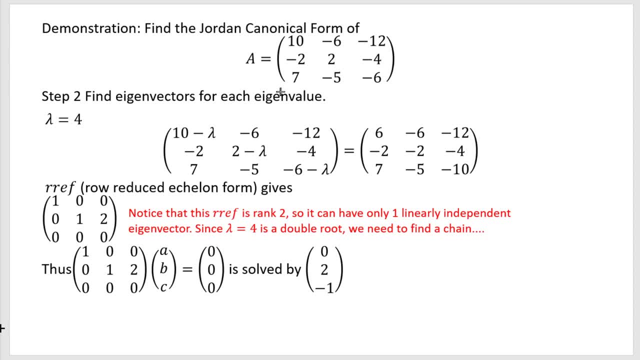 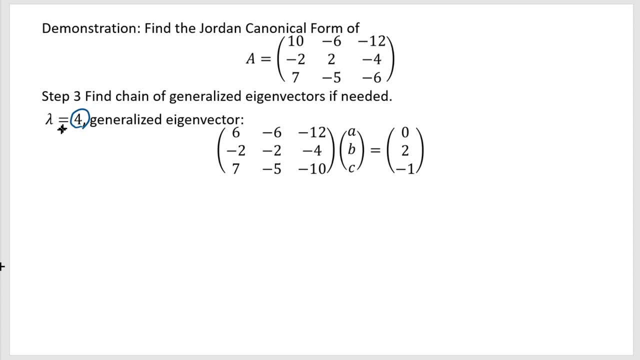 So we immediately know that you can't diagonalize this and therefore you have to look for the generalized eigenvector. So since the eigenvalues were negative- 2,, 4,- and there was a multiplicity, there was another 4, and that's why we wanted two linearly independent eigenvectors for this value. 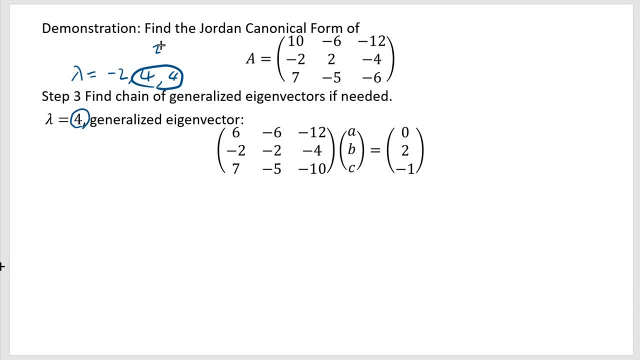 Okay, So in that case you have to find the generalized eigenvector instead. okay, So what's the generalized eigenvector? If you recall, we had it like this: It's like V2 equals to V1.. So, since we found the V1, is this one: 0, 2, negative 1, now we have to say this matrix: 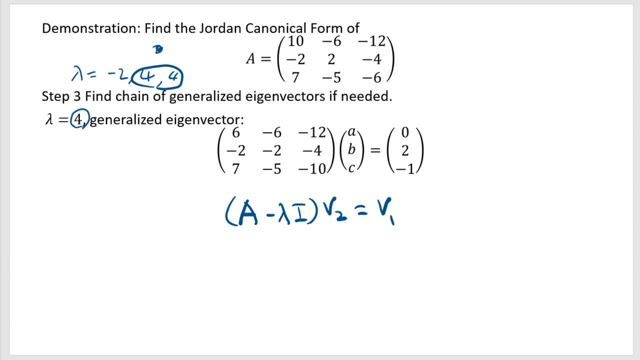 times this is equal to 0, 2, negative: 1.. Now, in that case, what you want to do? What you want to do is you want to build this matrix and do the row-reduced echelon form, and it goes like that: 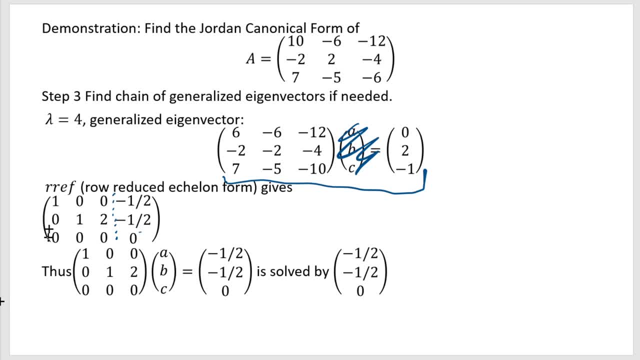 And it's really like this, so that this right side comes here. this is this. So solving the above equation is the same as solving for this row-reduced echelon form, which is like this one, And this is solved by: if you actually do the math, then this says: 1 times A equals. 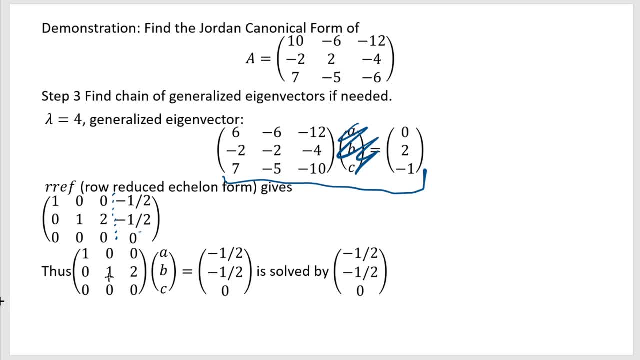 negative 1 half. So A has to be negative 1 half, And then B plus 2C has to be negative 1 half. And there's a choice, because you have one equation for two values of B and C And I just chose C to be 0, so that B would be just negative 1 half. 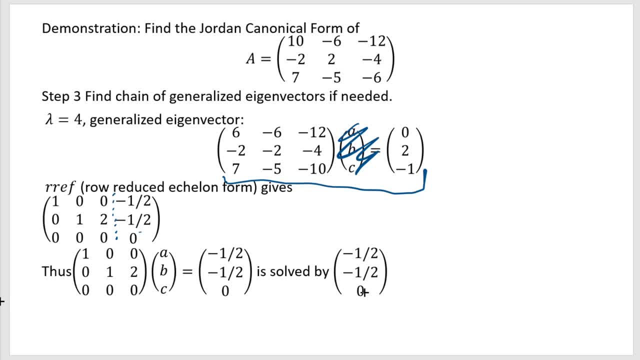 But you could have chosen some other values of C, but I don't see anything better by choosing other ones, So it seems to me this is the simplest. Okay, so we choose that as our chain, And now we're good to go. 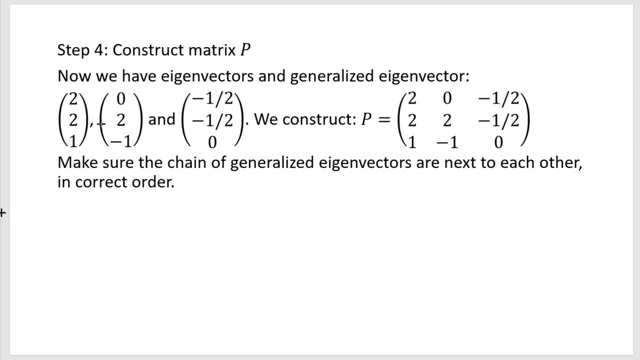 Because I have three linearly independent eigenvectors and also a generalized eigenvector And you put them together to construct P, And when you do this it's important that see V2 times A minus lambda, I is V1.. So V1 and V2 should be right next to each other. 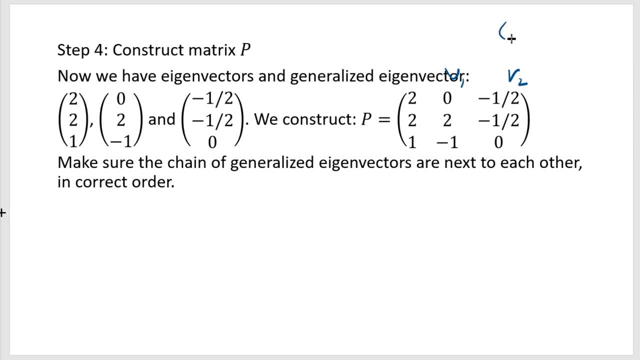 And if you had a third one, so A minus. if there was like A minus, lambda, I times, V3 equals V2, then it has to be in the order of V1,, V2, and V3 right next to each other. 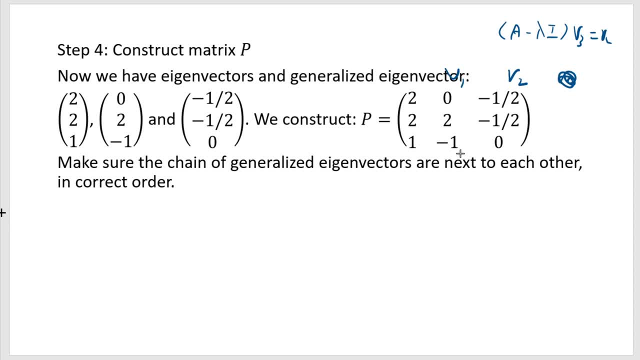 If you don't do that, then the final shape doesn't look like a Jordan form. I mean, if you're curious, you might try to switch these two and you'll see that, instead of the Jordan form, which is upper diagonal, upper triangular, you will see that you get. 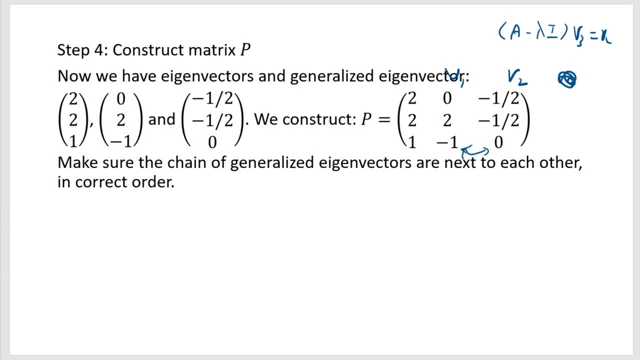 the lower triangular one. Okay, So that's something you can think about. Okay, All right, So you do that, And then what you want to do is you want to compute AP. This was our original matrix A, And we just build this matrix P And we got this. 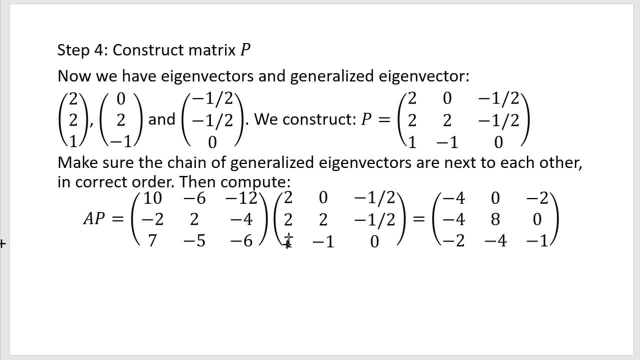 And you can actually do the calculation. but it's also true that, since this is an eigenvector of this thing with eigenvalue negative 2, negative 2 times this entire thing will give you that Okay. And also, since this one is an eigenvector with eigenvalue 4, this times 4 will give. 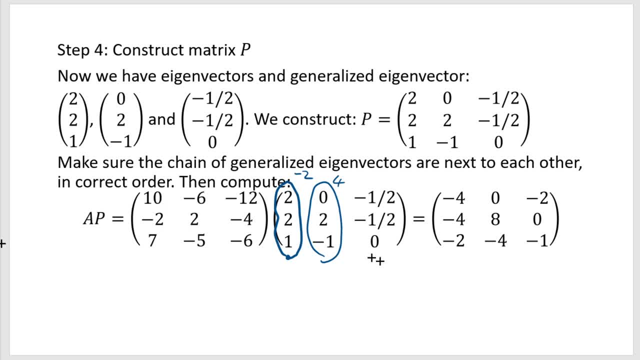 you this, And if you don't trust me, you can actually do the computation and you will see that you get exactly 0,, 8, negative 4.. And finally, this one is an eigenvector of eigenvalue 4, but you know, A V2 is equal. 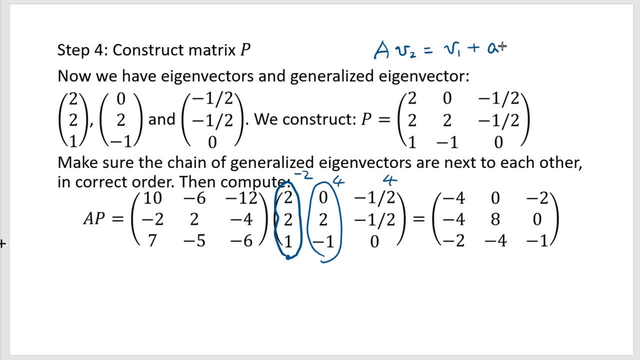 to V1 plus A lambda V2.. So that's the 4, 4 times V2.. So multiply by 4 of this, But you have to add the V1, which is this one, And that's why you get this. 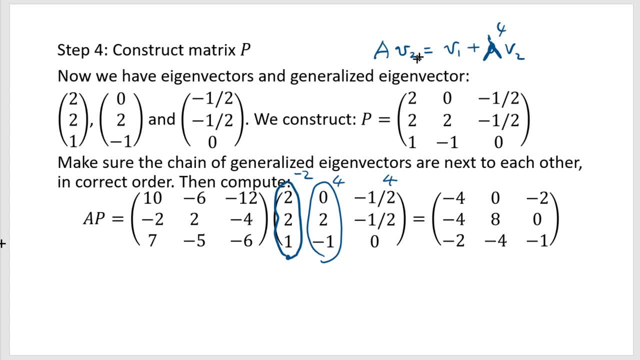 Okay, All right, So you can do the shortcut and get this one, or you can actually do the multiplication honestly, But whatever you do, it's this one. Now you can check that. the above is same thing as P times this Jordan canonical form. 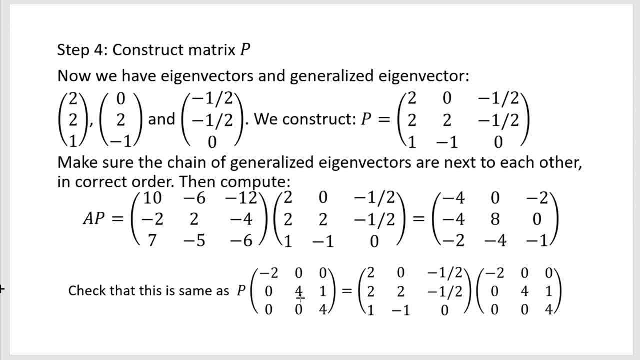 where you have negative 2 and 4.. Those are the two eigenvectors, but eigenvalues. but there's this 1, because this is the block diagonal And if you look at the mechanism, how this works, you see that, indeed, when you multiply,